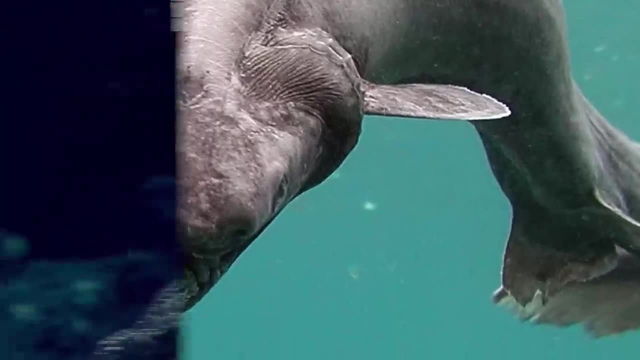 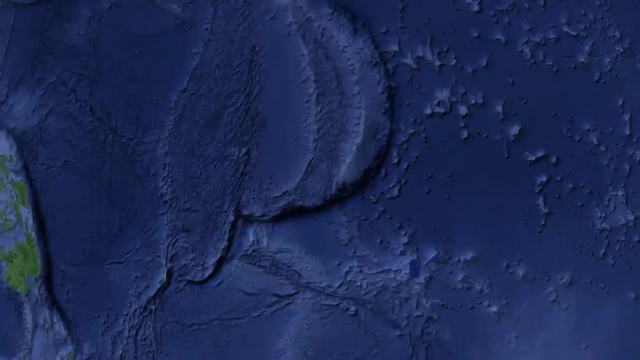 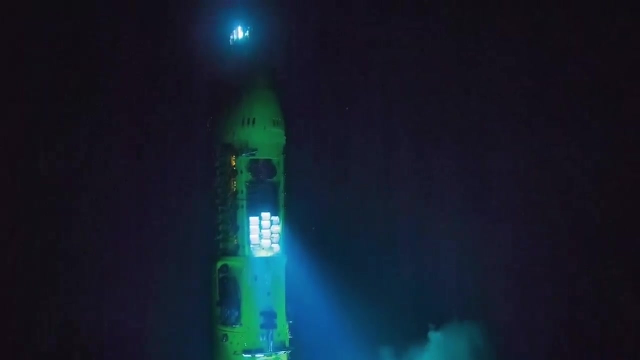 scar over 1,500 miles long, cut into the crust of the earth And, at the bottom of the Mariana Trench, the deepest known point on earth, named the Challenger Deep. It is over 36,000 feet deep If you drop the highest mountain on earth, Mount Everest, into the Challenger Deep. 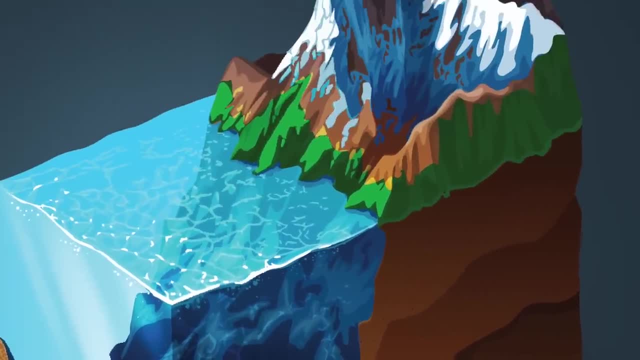 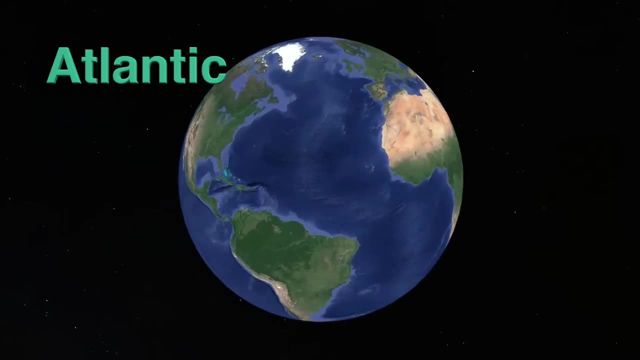 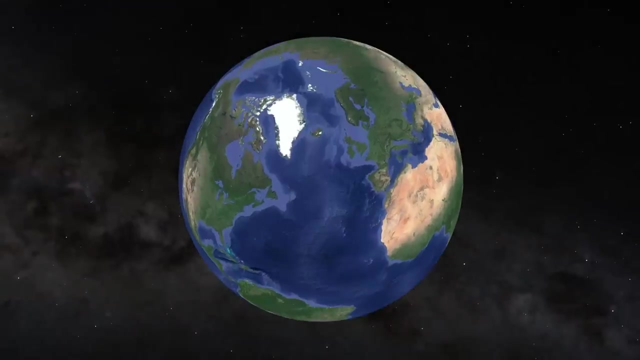 it would still be covered with over a mile of seawater. That's deep. The next ocean is the Atlantic Ocean. Although the Atlantic is number two, it is gigantic. Like the Pacific Ocean, the Atlantic Ocean also reaches north to the Arctic Ocean and down to the Southern Ocean. 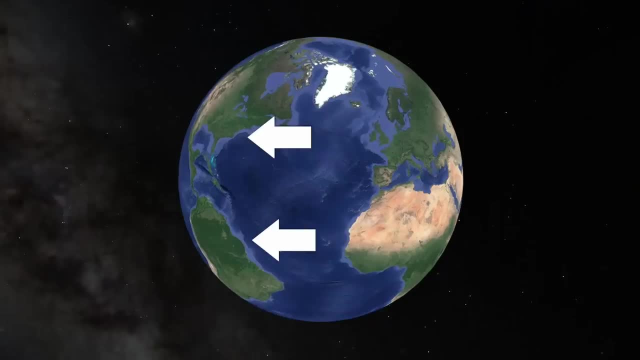 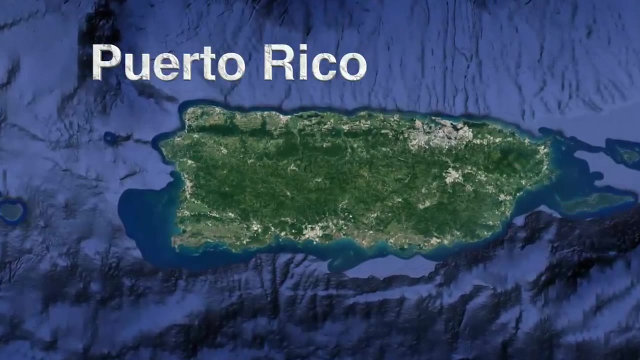 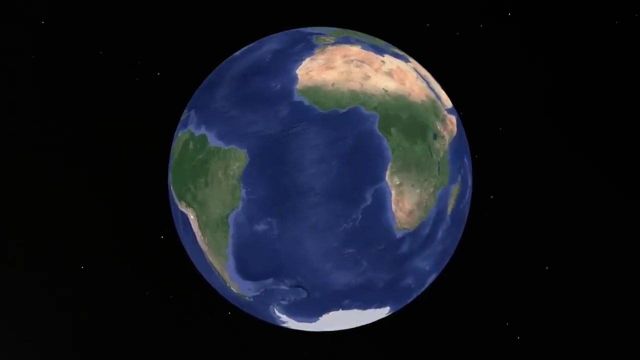 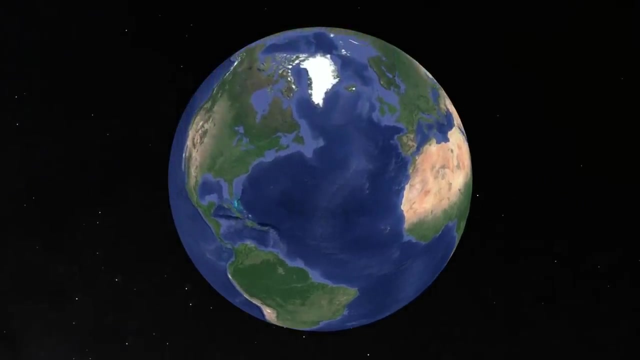 and borders, North and South America- And then it reaches far across over to Europe and Africa. The island of Puerto Rico is in the Atlantic Ocean. The Atlantic Ocean kind of looks like an S as it follows the coasts of its borders And it separates the old world of Europe and Asia and Africa from the new world of the Americas. 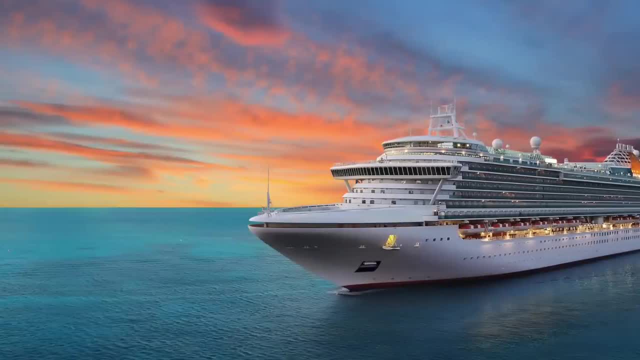 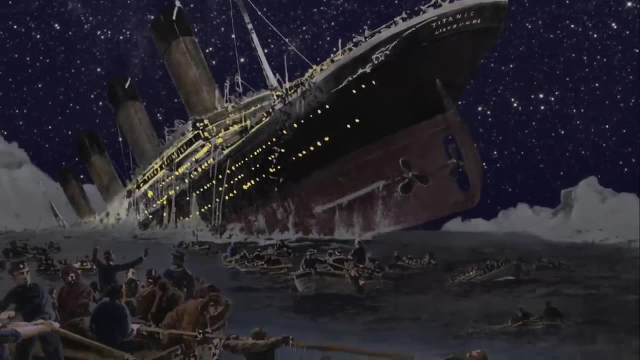 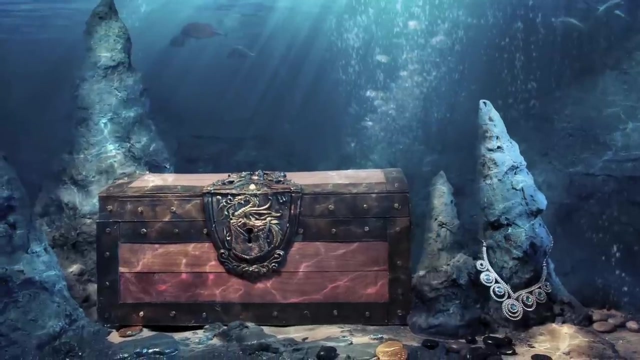 Over the thousands of years, many thousands of ships have crossed the Atlantic And thousands of ships have sunk in the Atlantic. The Titanic hit an iceberg in the Atlantic and sank. Many ships still with valuable treasure are scattered all over the Atlantic Ocean waiting to be found. 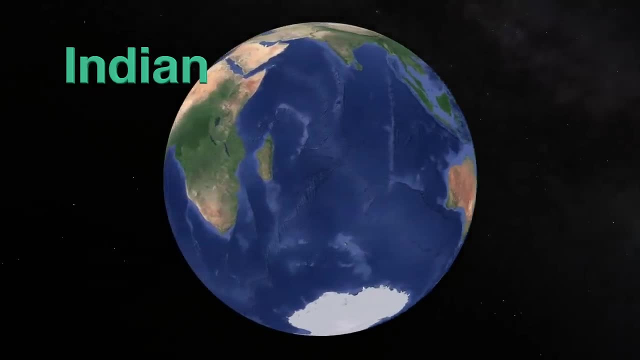 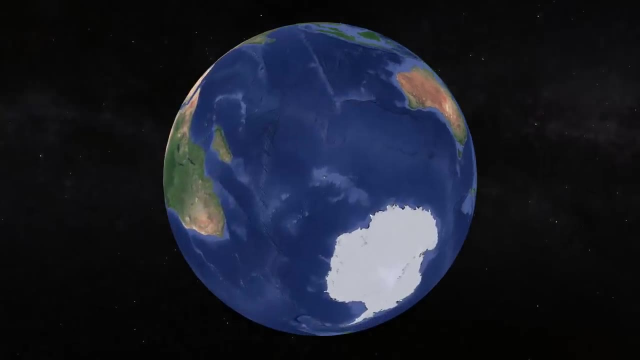 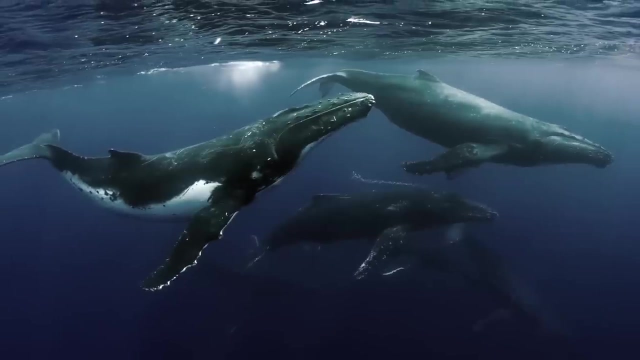 Ocean number three, the Indian Ocean. The boundaries of the Indian Ocean are Africa, Southern Asia, Australia and the Southern Ocean. The Indian Ocean is the largest breeding ground for the humpback whale, But it is also the source for a large percentage of oil pumping. 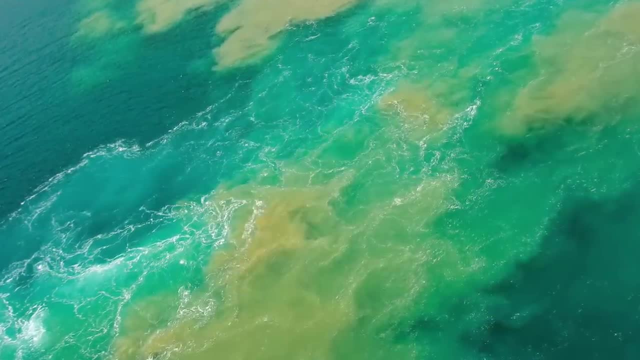 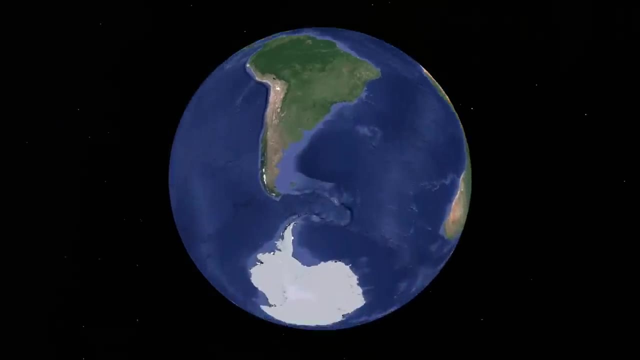 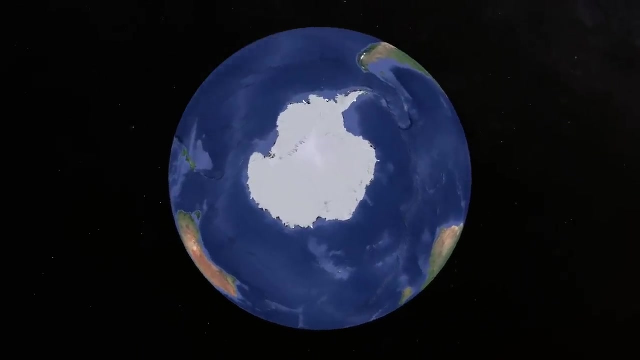 Oil spills are believed to be a great threat to the health of the Indian Ocean and the life in the ocean. let's consider the southern ocean, also known as the antarctic ocean, which waters encompasses the southern continent of antarctica and touches three oceans of the world. 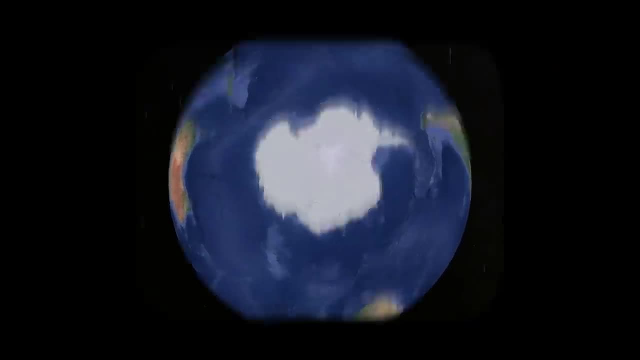 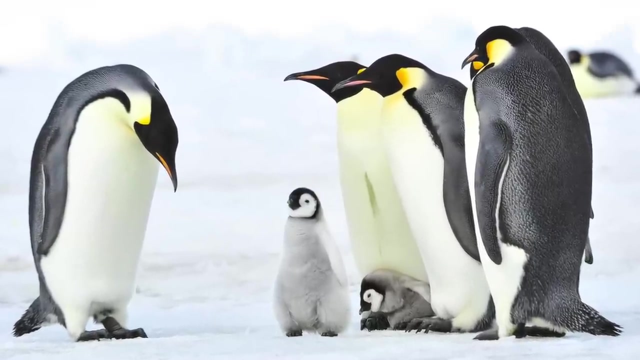 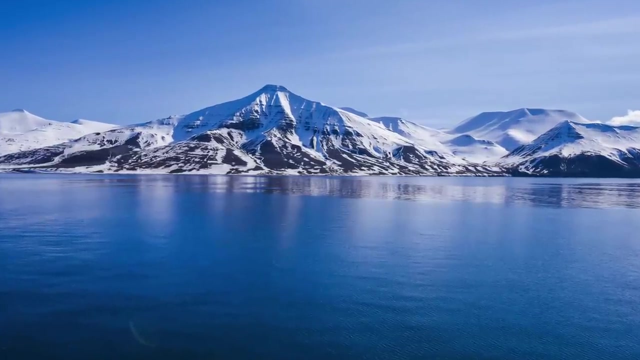 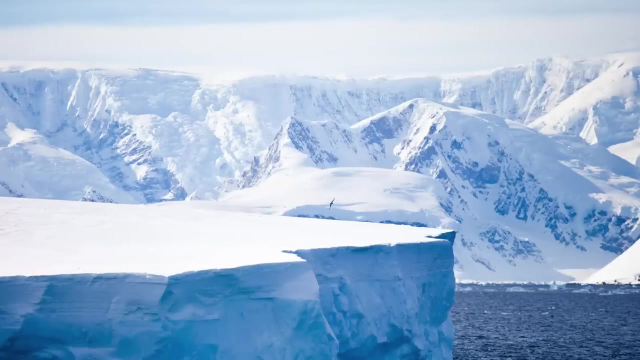 the pacific, the atlantic and the indian oceans. the world's largest penguin species, the emperor penguin, live on the ice of the southern ocean. did i say ice? yes, ice. the southern ocean is cold. it's the coldest ocean because of the sheet of ice that covers antarctica. it's cold all the time. this brings us to our last-named ocean. it surrounds and covers the north pole, where there is no land but only ice and ocean water, and this ocean is named the arctic ocean. the arctic ocean may be the smallest of our oceans, but it's not small. it is very, very large, and during the warmer months, some of the ice melts and becomes ocean water, and during colder months, the water freezes and becomes ice. 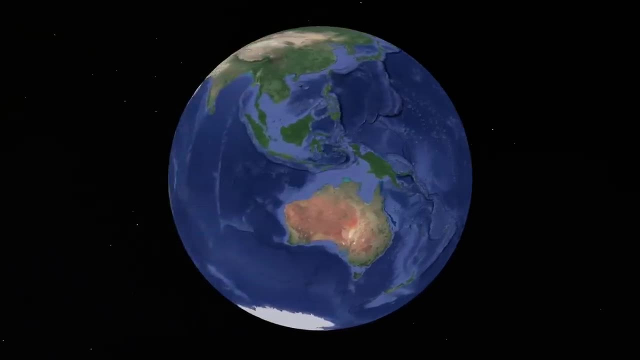 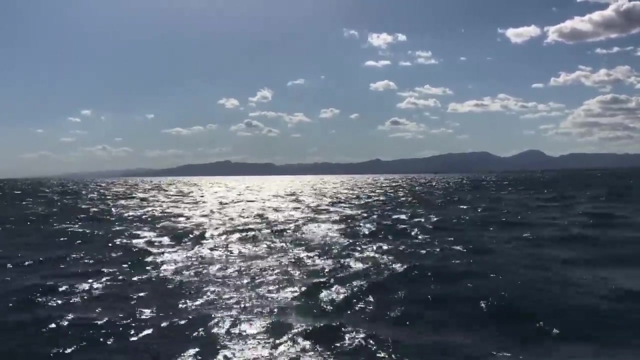 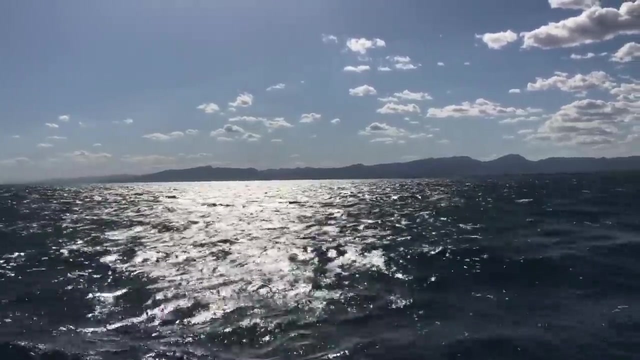 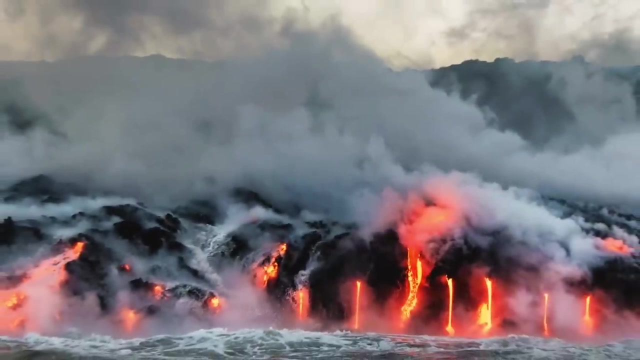 these are the five oceans of the world. as you look out over these waters of the ocean, you may think i can't see anything over the water and i can't see under the surface. there must be nothing there and you may think nothing is going on down there, but the truth is a lot is going on in the ocean. there are volcanoes in the ocean. 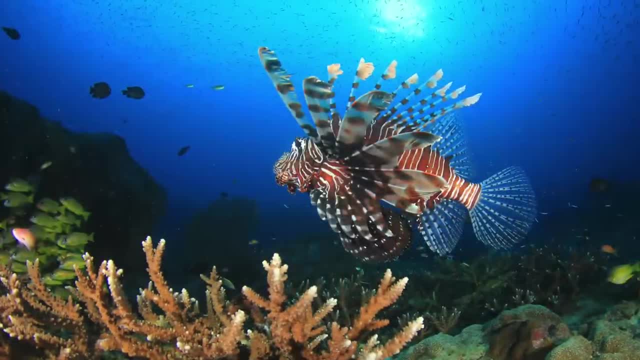 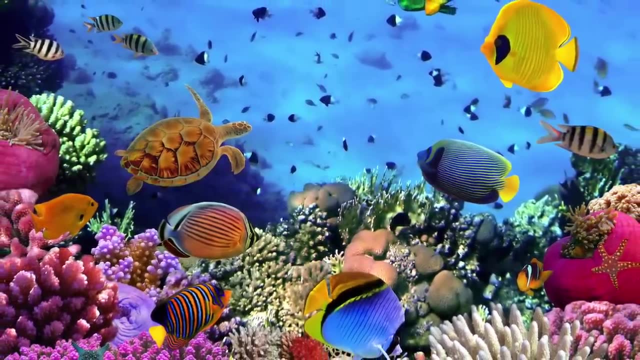 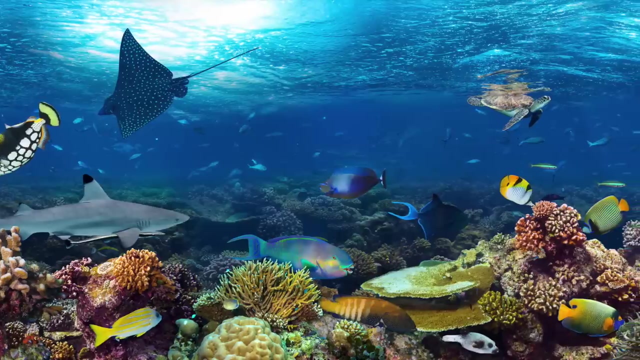 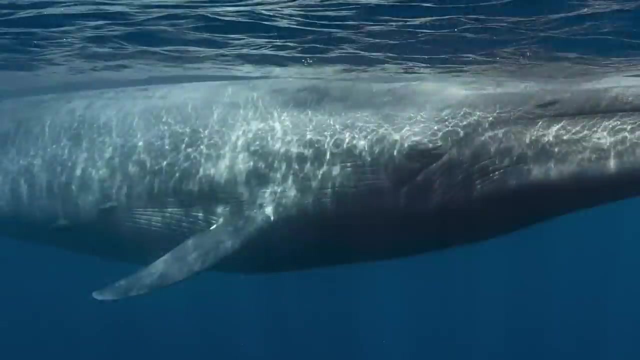 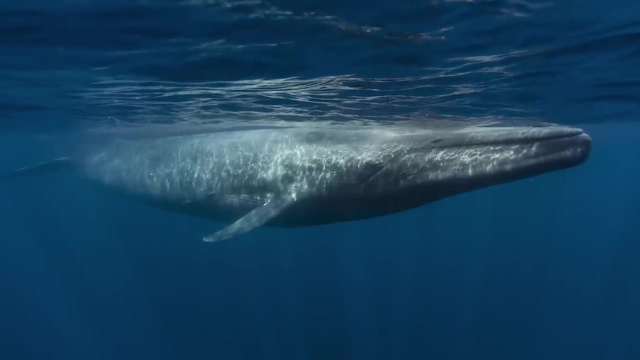 volcanoes spewing lava and life living living things are in the ocean. hundreds of thousands of species of animals and plants are in the oceans of the world, from the coldest waters of the ocean to the warmest. many varieties of animals make the oceans their home, from the tiny krill to the largest animal on earth, the blue whale, they make their home in the oceans. plants and animals rely on healthy, clean seawater to survive. 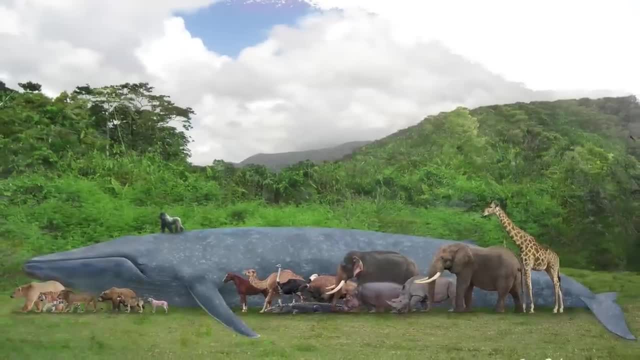 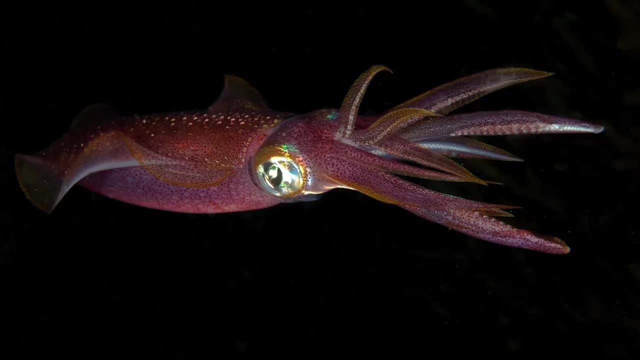 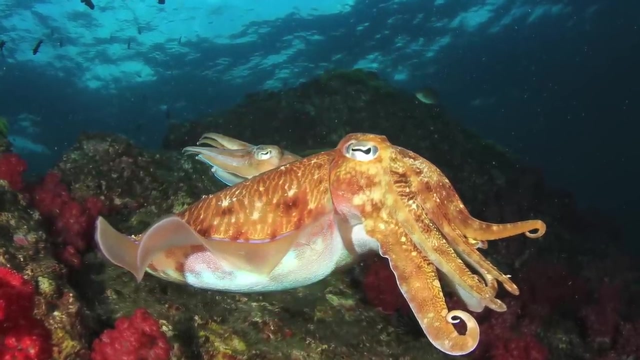 and thrive. i don't think a blue whale would walk very easily on land, do you? strange and freaky looking animals like octopus and squid and the nautilus and the cuttlefish? these amazing and intelligent creatures live in these waters as well. fish of every shape and size and color. 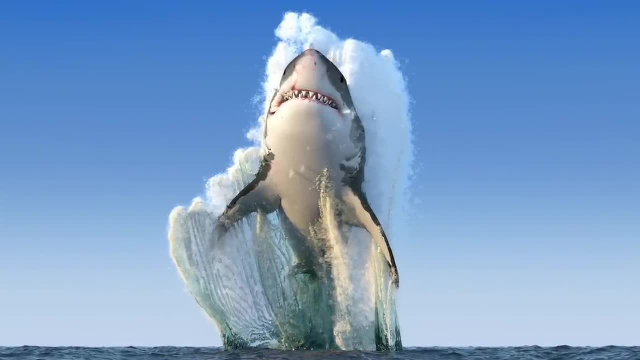 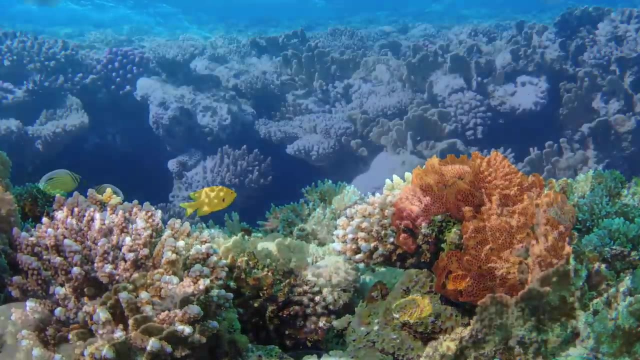 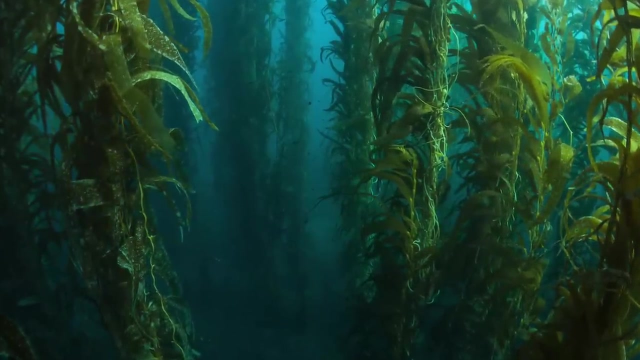 and sharks. they are down there. what do you think you'll find on the ocean floor? if you say gardens of spectacular quality, coral reefs which grow very slowly, and plants and sponges that grow and provide protection for smaller critters, well, you'd be right. In deep way, deep down in the ocean, where light cannot.